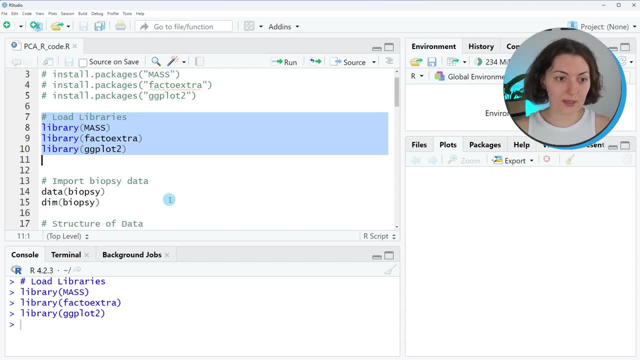 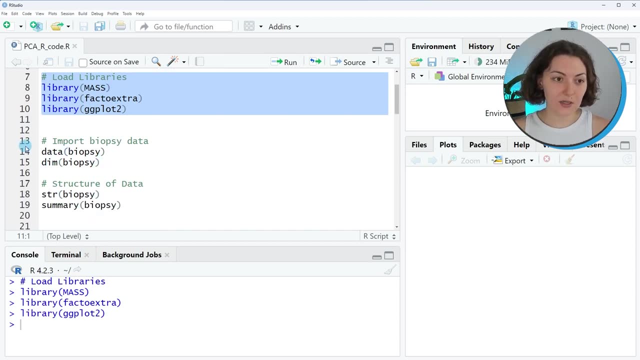 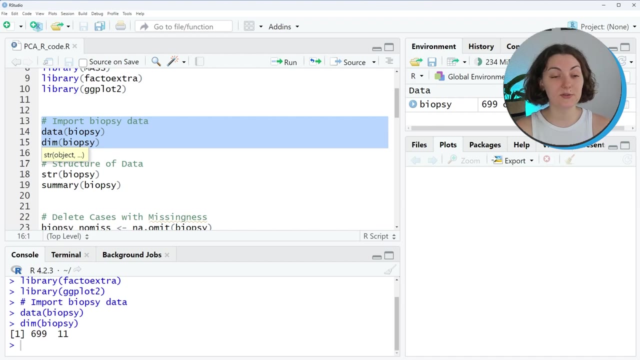 as follows. And after this step, you can import your data. We will import the biopsy data from the mass package, So let's do it. This data contains biopsies of breast tumors for 699 patients and, relatedly, you can see that the data set has 699 rows and 11 columns. 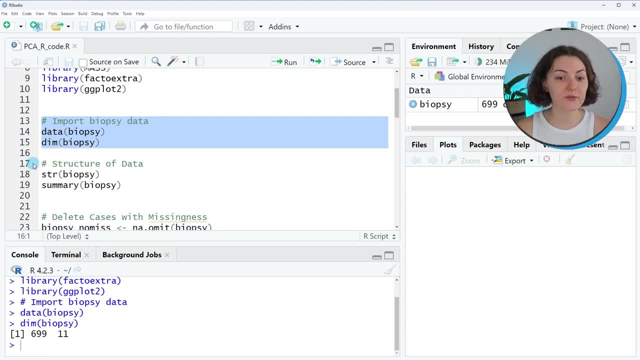 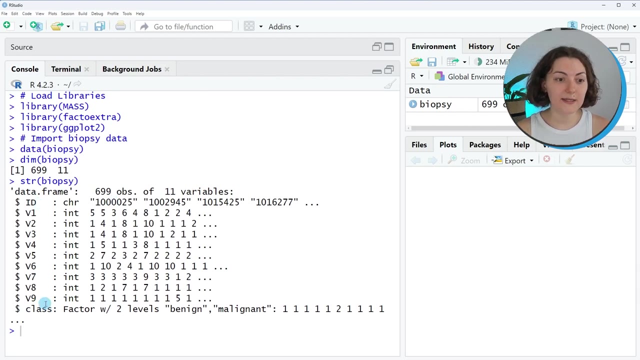 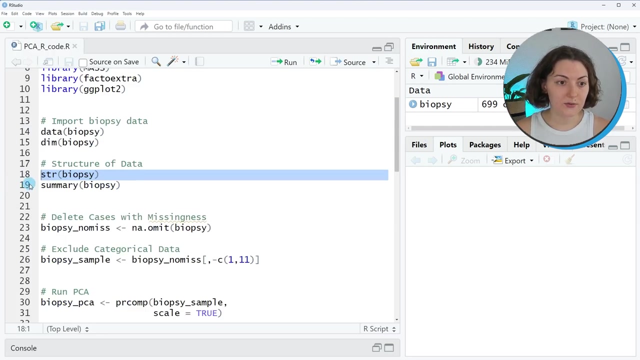 I will also use the CTR function to observe the variable types which matters in PCA. So let's run it. As you can see, except for the ID and the class variable, all variables are numeric as desired. I can do a further investigation by running the summary function. 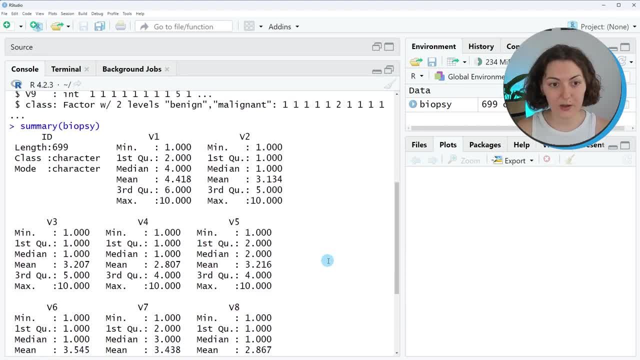 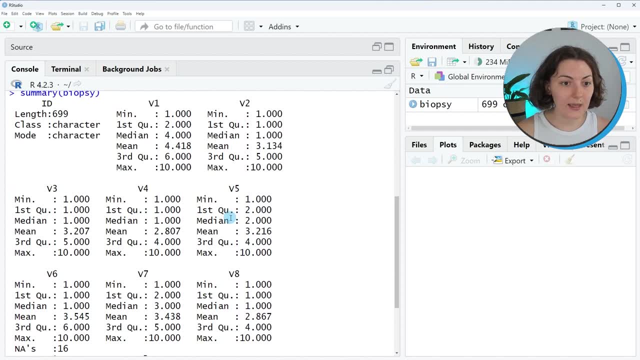 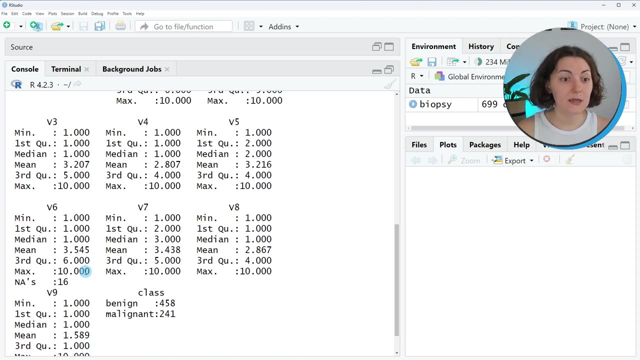 And it gives more detailed information about the variables and you can see that the numeric variables are ranged between 1 and 10, and also it shows that we 6 have 16 missing values. and also you can see the partitioning of categories in the class variable and so on. 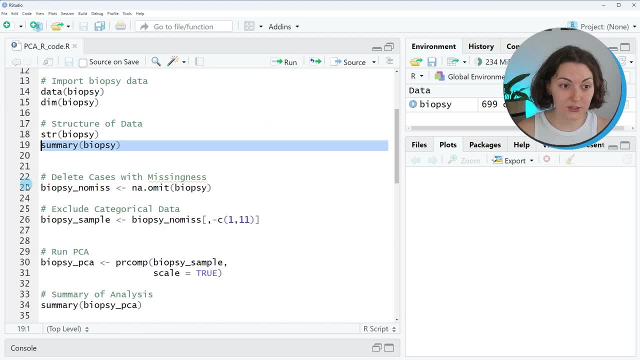 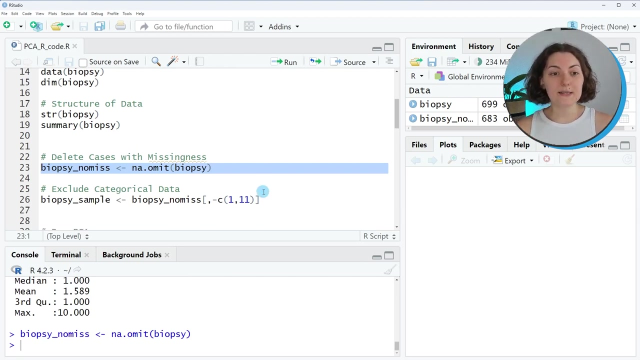 so, based on this information, first, i need to deal with missingness in this tutorial. i will use a listwise deletion to keep it simple, but usually it's not the best approach concerning bias and information loss and so on, and so let's also run this now. i omitted the cases with 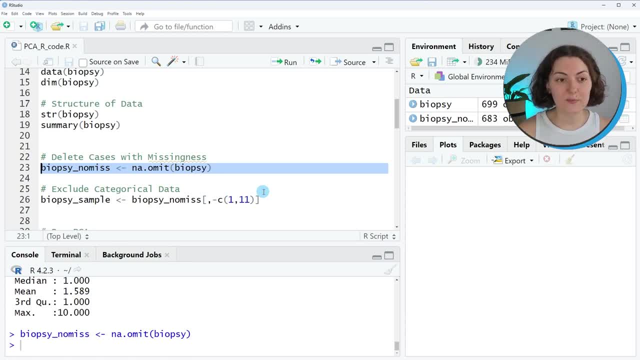 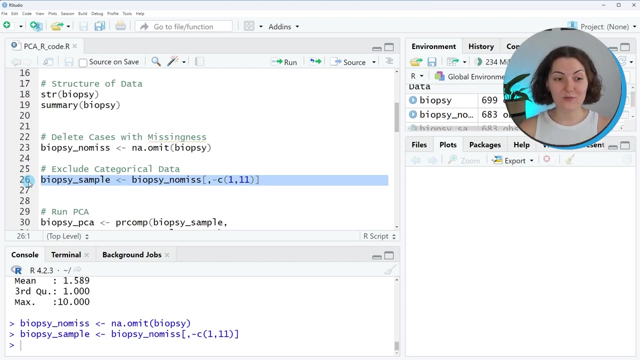 missingness and i renamed my data as biopsy. no miss. the second data manipulation will be about discarding the categorical variables which were in the first and in the last column. so and i will rename the data as biopsy sample and this will be the final data that i will use in 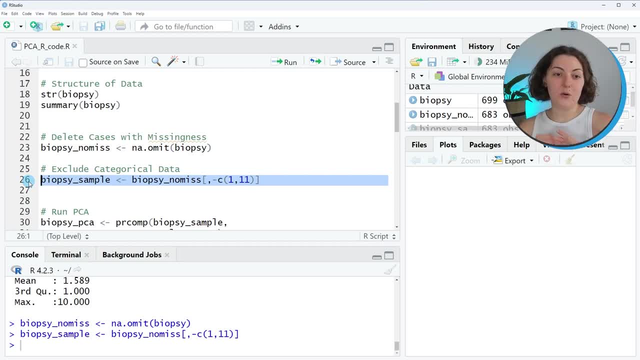 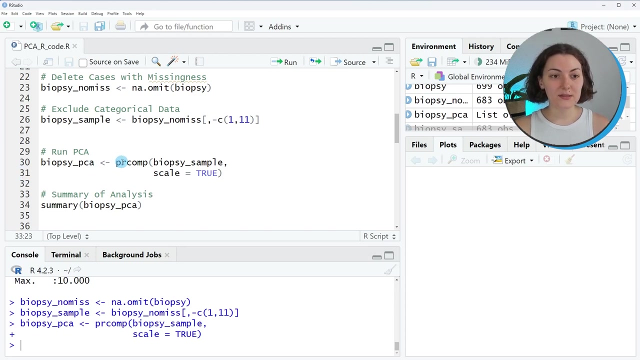 the principal component, analysis. if you want to learn more about why we- why we- discarded the categorical variables, you can check our tutorial on statistics globe called can pca be used for categorical variables? since now our data is ready to go, we can run the pca. we will use the pr com function to do it, setting the scale argument true, which ensures that 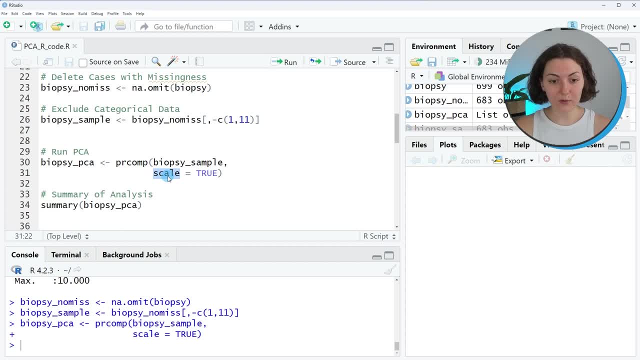 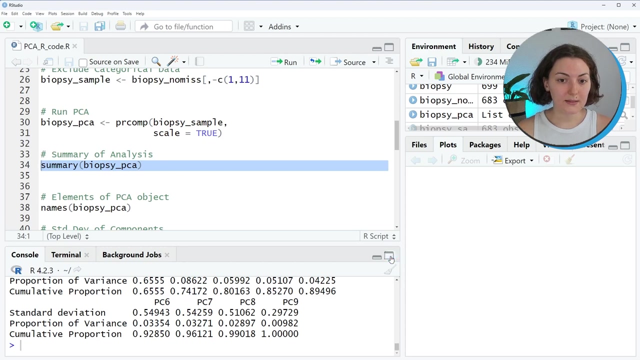 our data is standardized, it is important to avoid bias in our analysis. for further information, you are welcome to check our tutorial on statistics globe pca using correlation metrics versus covariance metrics. so let's run this. and now our analysis is conducted, we can print the summary, and this summary gives: 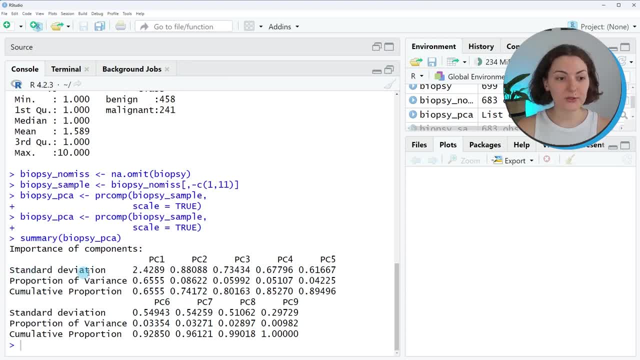 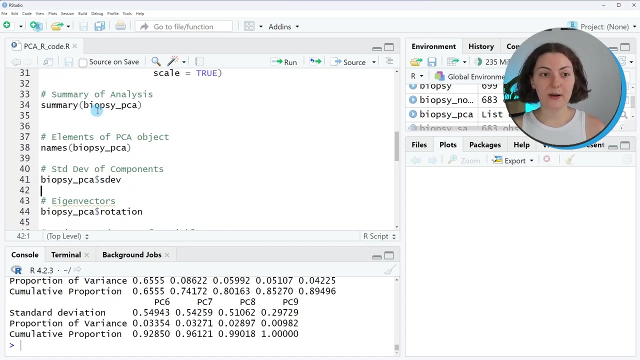 the importance of components. so in the first row you'll see the standard deviation per component, in the second row you'll observe proportion of variance per component and the last row is the cumulative sum of the second row. all right, now let's check the other data saved in the pca. object: biopsy, pca, and we can check what. 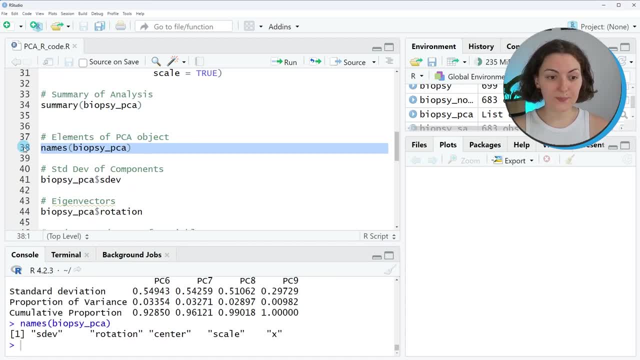 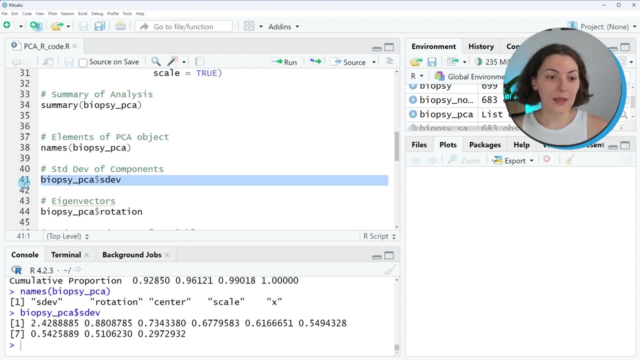 they are by calling the names function. so you see that there are five more elements providing some additional analysis output. the first one is the standard deviation of components and the second one is called rotation. but it's not called rotation, but it's called the result of the. 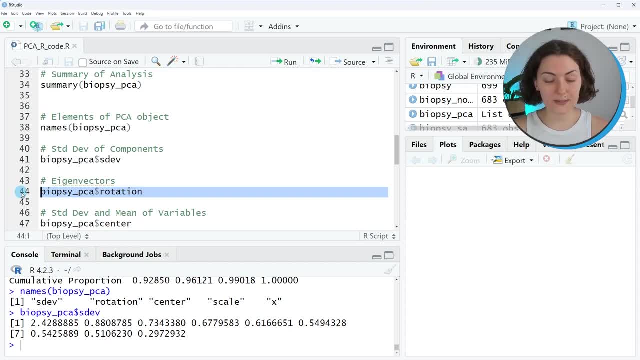 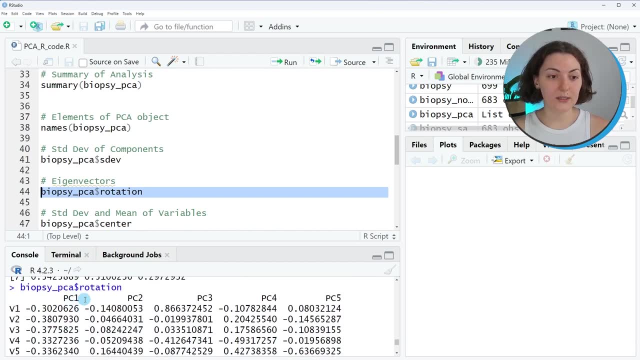 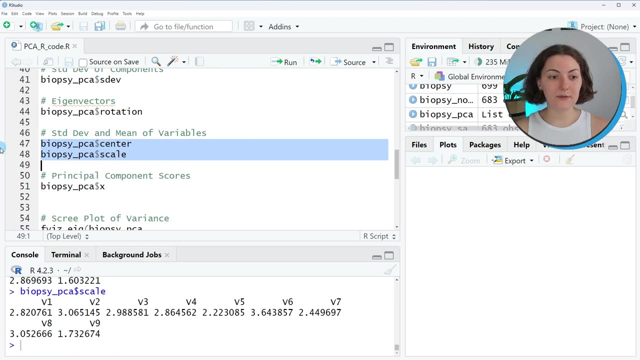 it's actually provides the eigenvectors, which contains the loadings per variable, per component, and the third and the fourth elements are the mean and the standard deviation of the original variables. these are the values used in the standardization, in this analysis, and the final element is the principal component values. 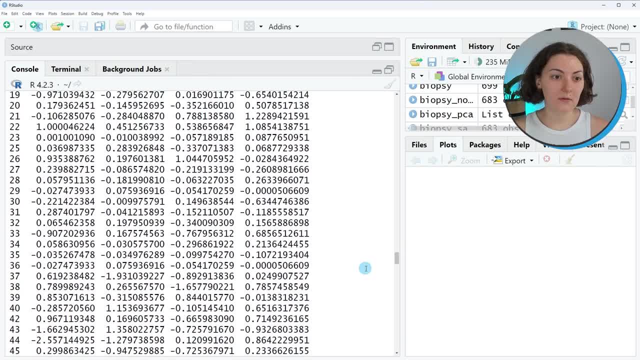 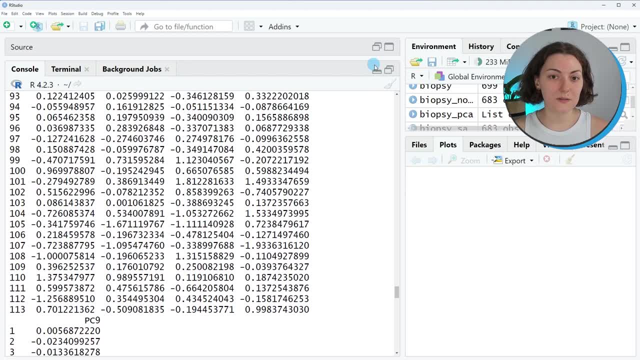 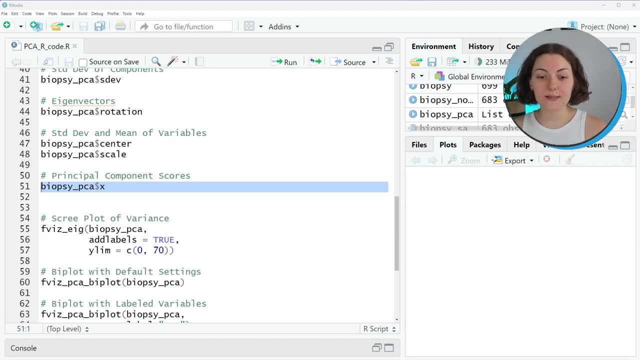 let me show you like this principal component values, also called principal component scores, for all nine components as shown, all necessary information and stored in the pca object. in case of need, you can retrieve and do some further computations using them. now i'll show you how to visualize these results. uh, thanks to the factor extra package. you don't. 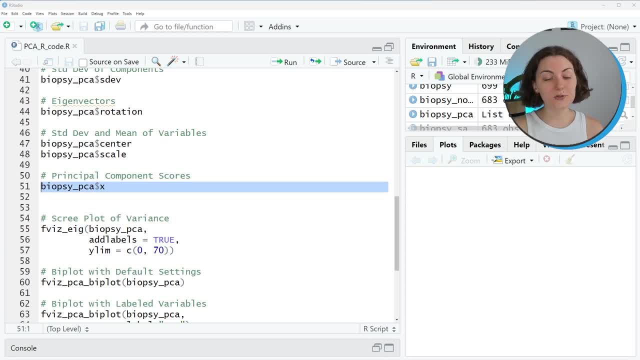 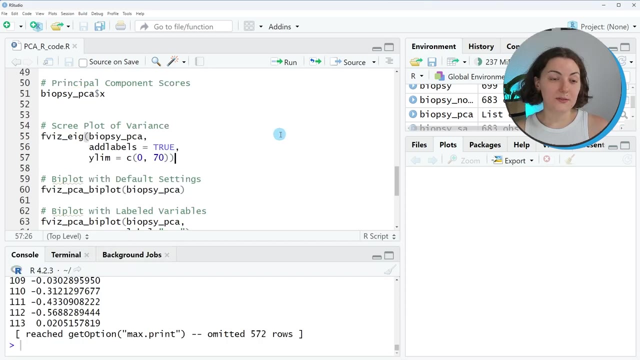 need to parse these stored elements manually to a function to visualize your results. instead, you need to just plug your pca object- which is a biopsy pca in our case- and into the specific function of factor extra package. so let's take the scree plot. it's a plot. 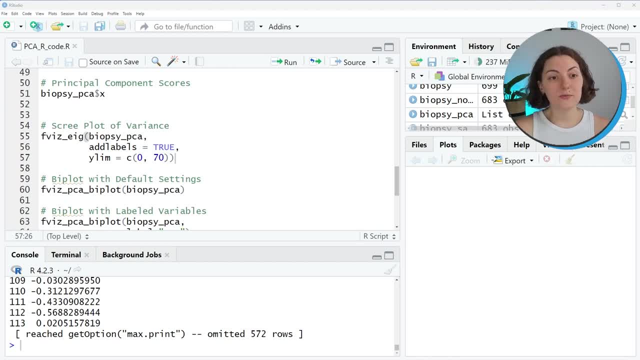 that shows explain variables per component. we use it to decide on the optimal number of components to retain in the analysis. we will use the fx i function of factor extra to obtain this plot and, as seen, uh. first we will input the p, pca object and then um we will set the ad labels. argumental. 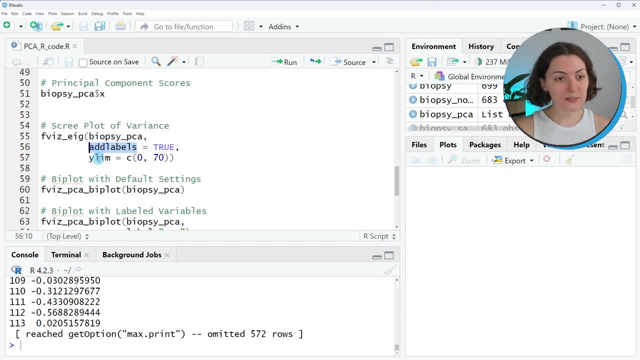 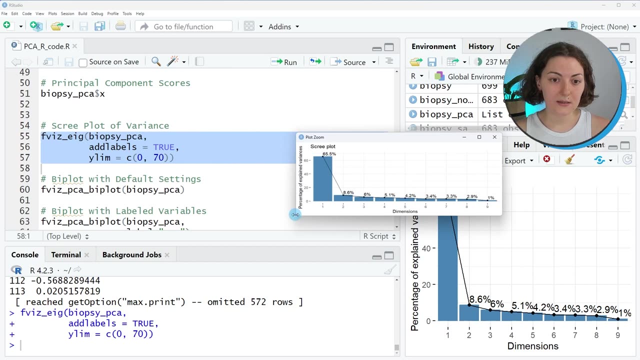 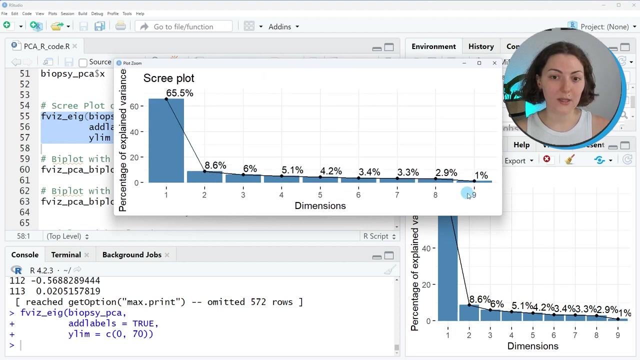 true to visualize the pca object, and then we will set the ad labels argumental. true to visualize the variance percentages. and you can also set the y-limb argument to arrange the limits of the y-axis. let's run this plot and, as seen, all percentages are shown for all nine components. 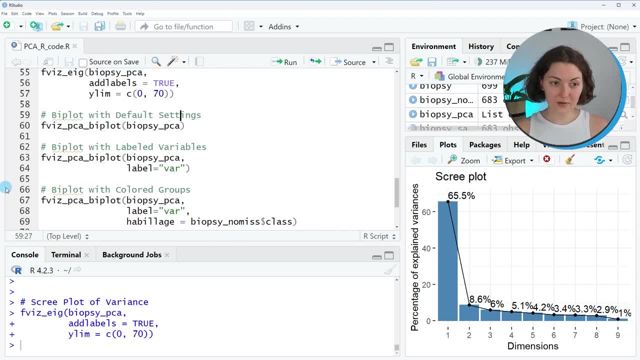 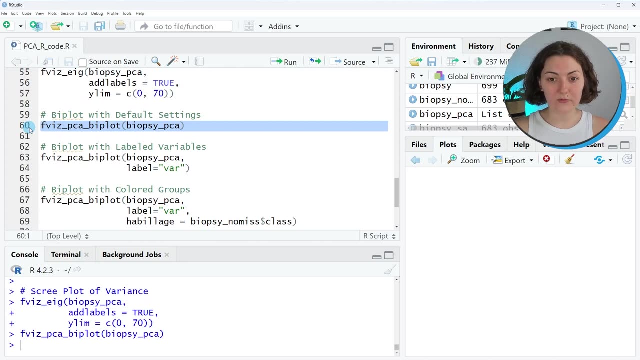 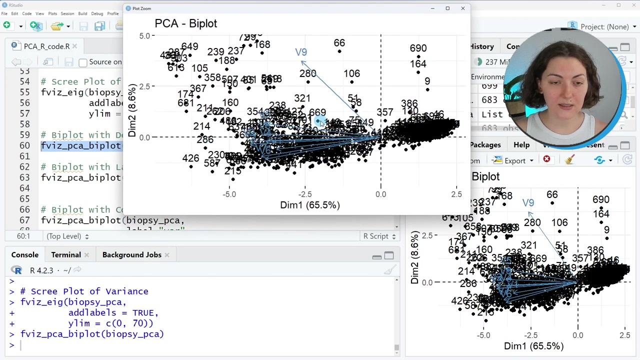 now we will continue with the biplot which is used to interpret the pca results, if its pca biplot function will be used. and, as you see, we input our pca object and when we run this we obtain the shown plot. you can zoom that in and see how all the 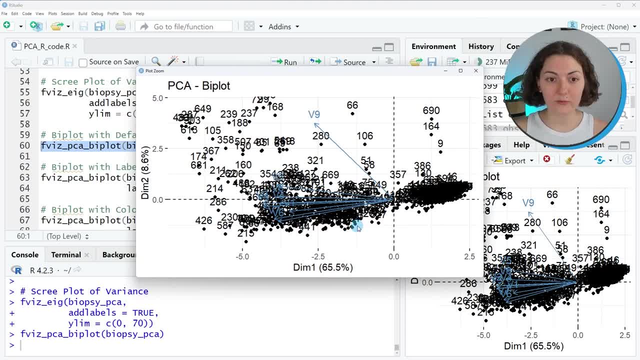 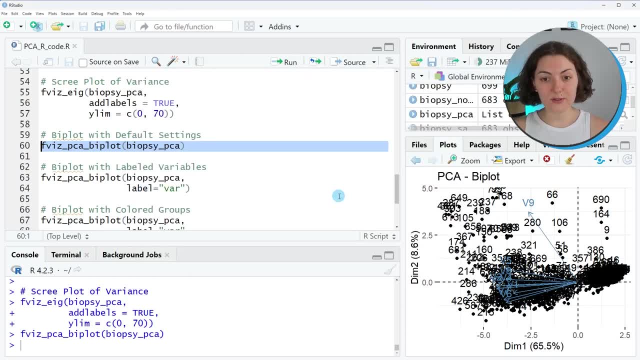 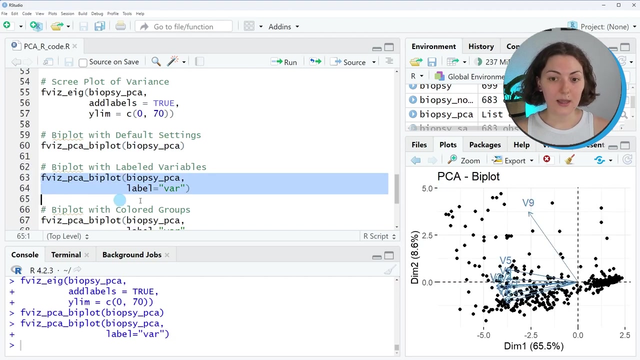 data points and values are variable, vectors are labeled by default. if you want to suppress the labels of the data points, which is usually preferred, since this view is a bit crowded, you can set the label argument to var, which which is all by default, and then rerun it, and now you will obtain.